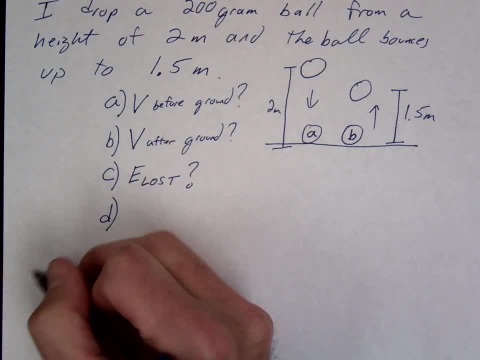 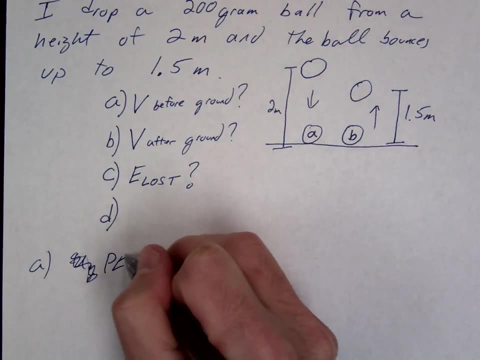 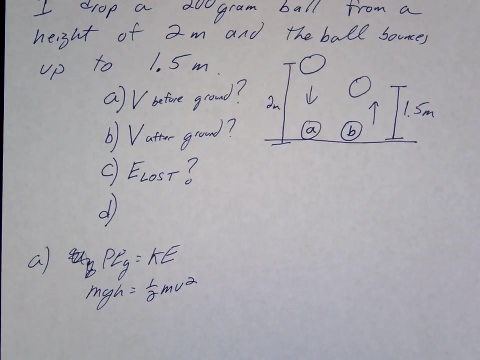 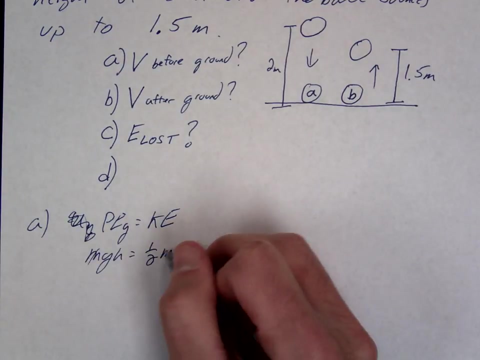 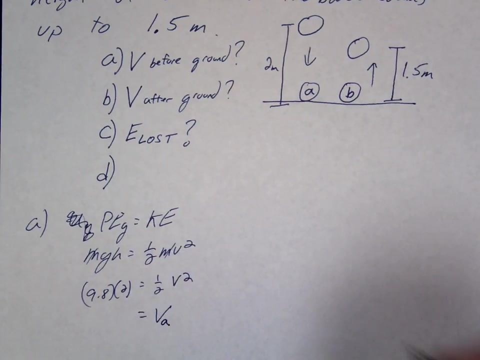 Okay, so letter A should be pretty straightforward, right? You just did that in the previous problem. It's just one of the simple PEs to KEs. Okay, so what are we getting for the V at point A? Okay, 6.26.. So that's how fast it's moving right before hitting the ground. 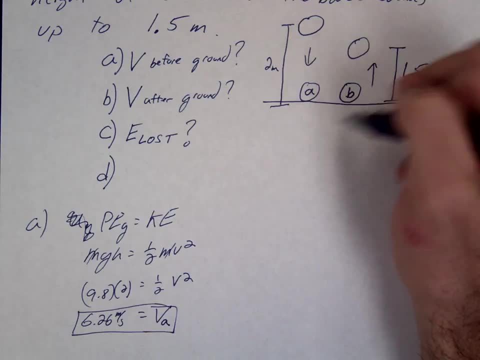 6.26.. 6 meters per second. Okay, then it's going to bounce back up. How are we going to solve for B? Yeah, Matt, Use 1.5 for H instead of 2.. Right, so we're bouncing up this way. 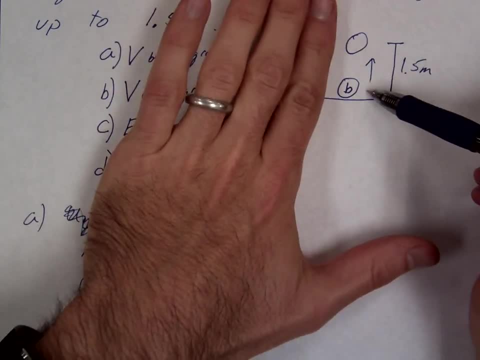 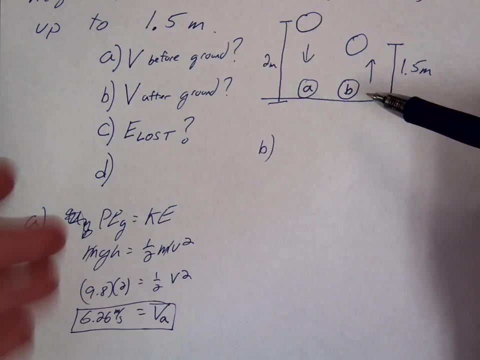 So we're just going to think of it. I mean, imagine I just said you threw a ball with some unknown velocity and it goes a height of 1.5.. How fast was it moving? Well, you would solve it in the same way, right? 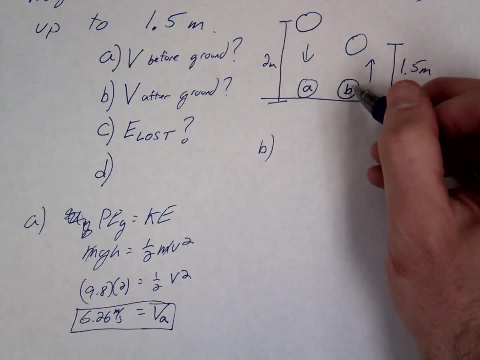 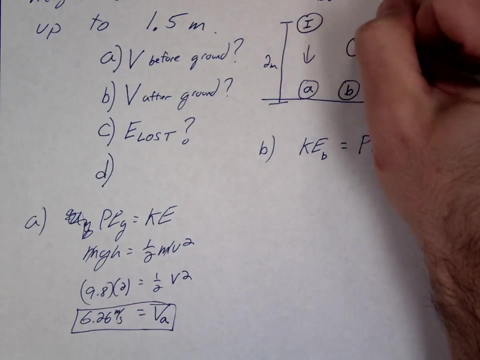 Except in this case. our E initial is right here, which would be kinetic. So we'd say, all right, the kinetic at point B should equal the potential at the top, or here Maybe we'll call this one the initial I, this one the final F. 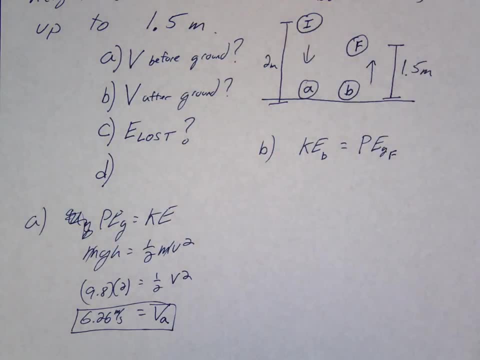 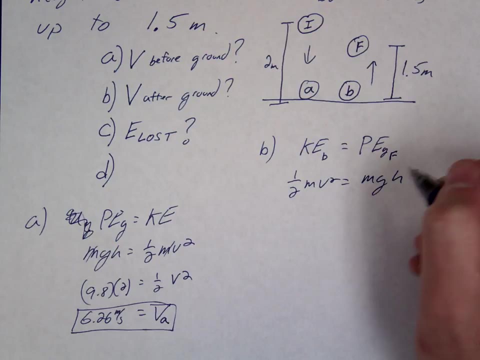 So what is the potential energy at the final? All right, so you just do it the same way, Except we use 1.5 for our height. Now we'll know we probably did it right, because what should be true about this V compared to this V? 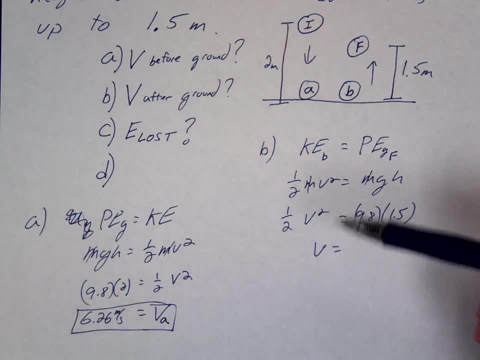 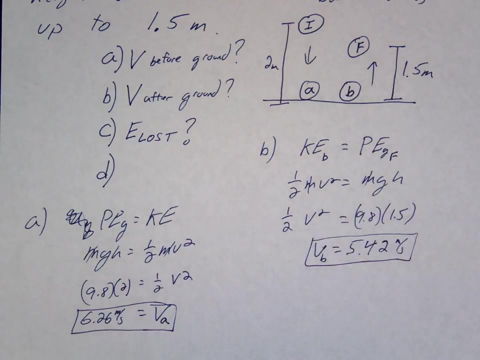 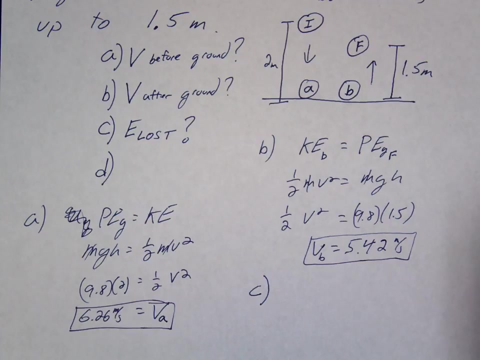 It should be less. right, It's not going as high, We're losing some energy. The V should be less, 5 point something, 4,, 3?, 2. So we'll call that VB, Okay. letter C: 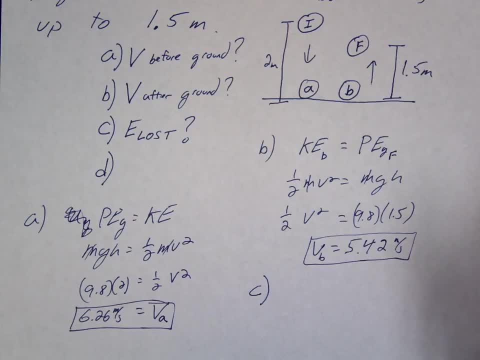 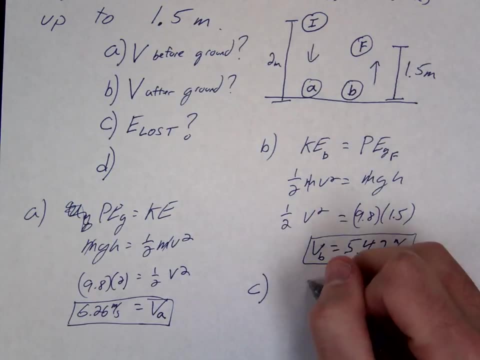 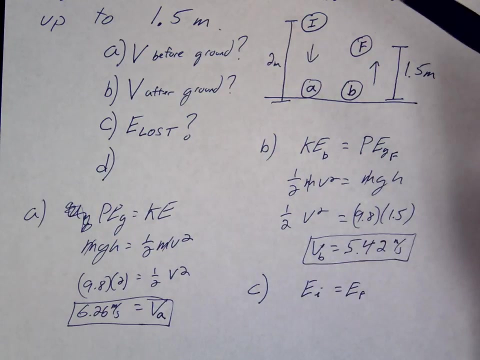 Energy lost. Okay, so at this point you actually have many options. You get many options to do it, So we are going to do E initial equals E final. The question is: what's our initial, what's our final? Well, you can make the initial here and the final here. 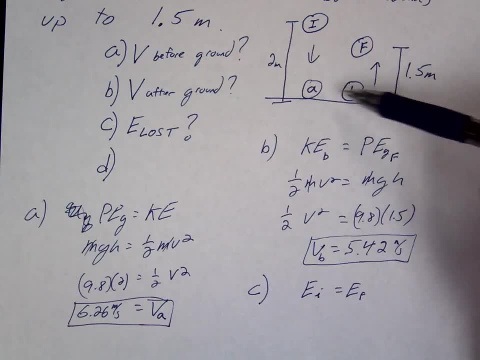 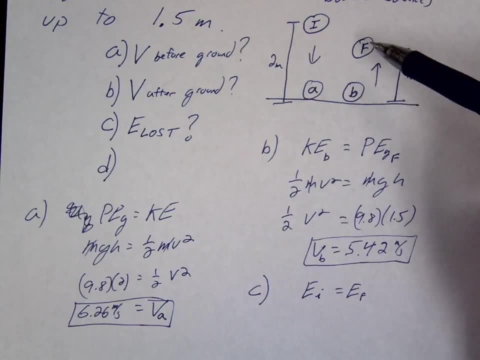 So between I and B, You can make it between A and B, You can make it between A and F, Or you can make it between I and F, It doesn't matter, as long as your initial is before the bounce and your final is after the bounce. 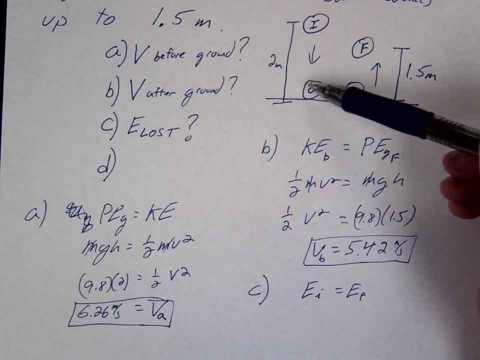 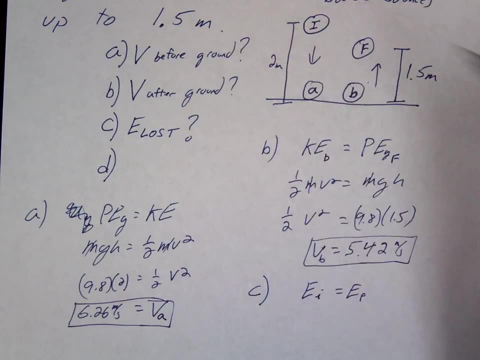 Most of the energy gets lost in the bounce, in the collision. So however you want to do, it is fine, You'll get the same answer either way. I personally like to just go from the very beginning to the very end, So that's how I'm going to do it. 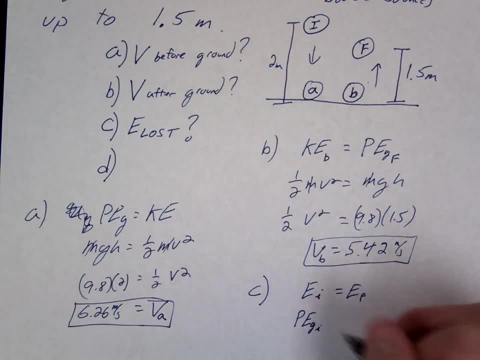 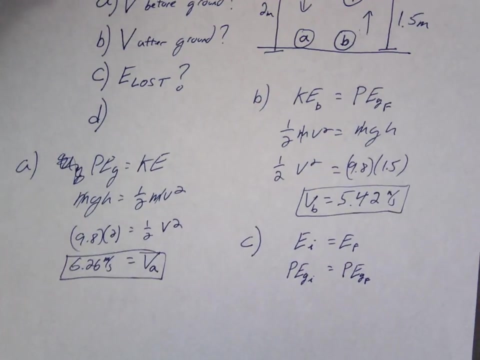 So I'm going to go: PE the very beginning, PE the very end, And then this is going to be less than this. right, We're going to start with more energy than we ended with, So we're going to add another term: elost. 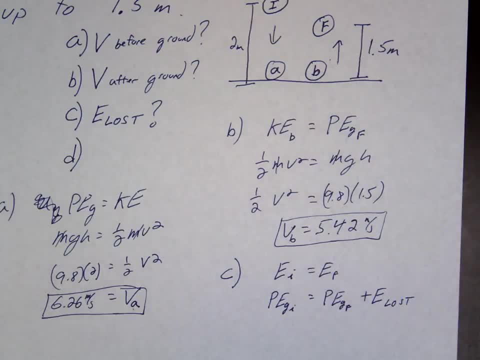 So mgh at the very beginning should equal mgh at the very end plus elost. Now be careful, you cannot cancel maths. Okay, Notice, it doesn't work. It's only in two of the three, Not all three. Okay, 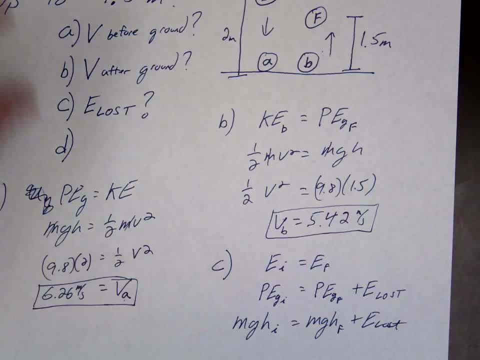 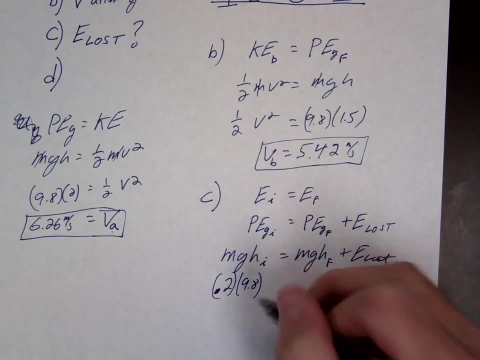 So 200 grams? what do we have to do with 200 grams? Convert that, yeah, So that's going to be 0.2 times 9.8 times what, was it 2?? And 0.2 times 9.8 times 1.5..